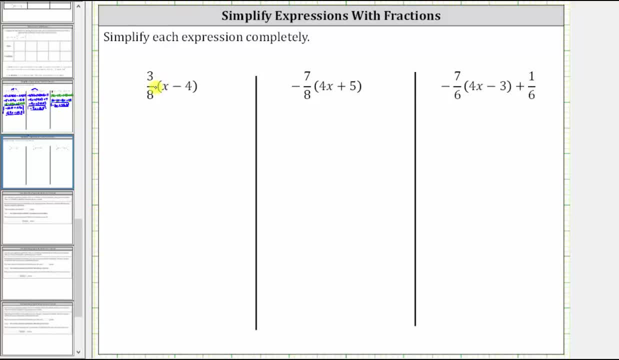 We are asked to simplify each expression completely. The first expression is 3 eighths times the quantity x minus four. We begin by clearing the parentheses by distributing 3 eighths. This gives us 3 eighths times x minus 3 eighths times four. 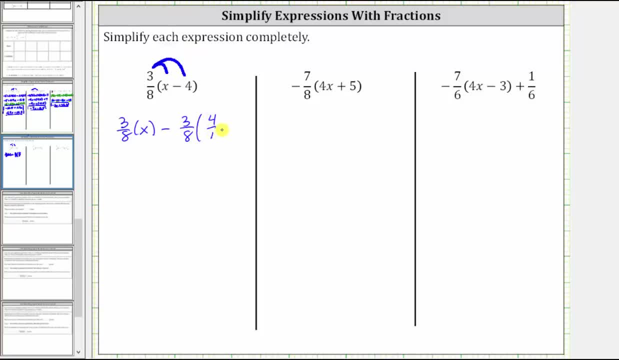 Let's write four as a fraction with a denominator of one: 3 eighths times x is 3 eighths x. Then we have minus Notice here. before multiplying, we can simplify: Four and eights are a common factor of four. 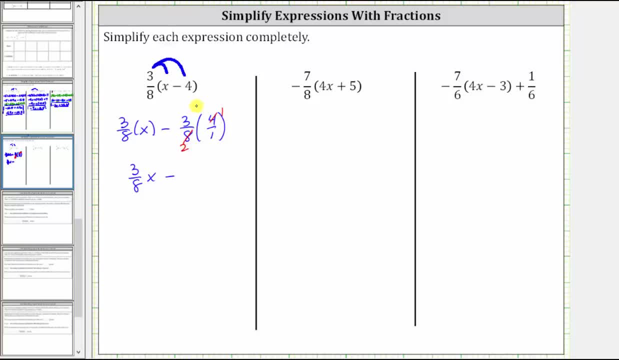 There's one four in four and two fours in eight. Multiplying the numerators and denominators, notice how here we get 3 halves, giving us the simplified expression of 3 eighths x minus 3 halves. Next we have negative 7 eighths. 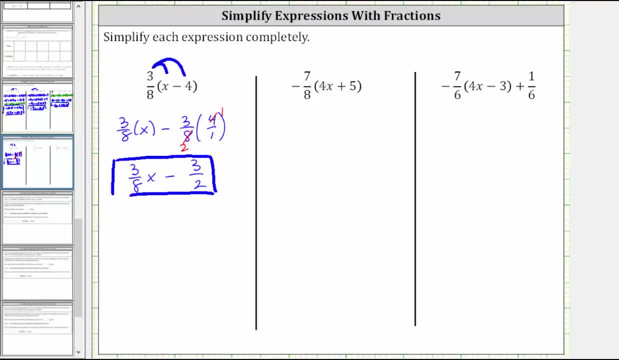 times the quantity four x plus five. We clear the parentheses by distributing negative 7 eighths. This gives us negative 7 eighths times four. x, which is a fraction, Can be written as four x over one, And then plus negative 7 eighths times five. 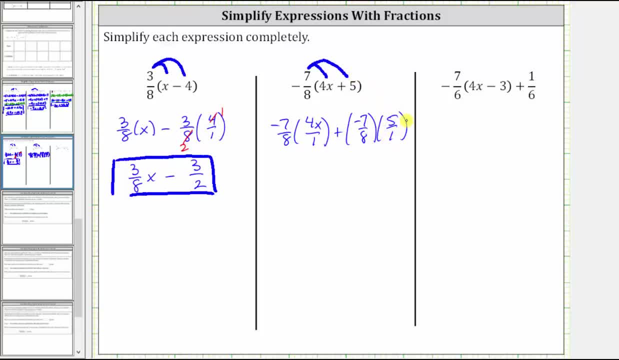 which, as a fraction, is five over one. Before multiplying here, notice four and eight share a common factor of four. There's one four in four here and two fours in eight here. Multiplying now, notice how we have negative seven x over two, which is equivalent to negative seven halves x. 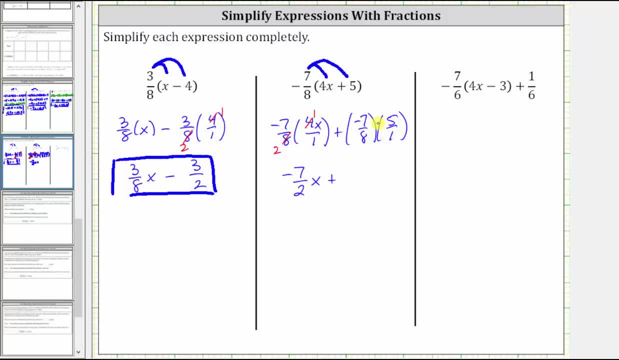 then we have plus. Nothing simplifies here. This product is negative 35 eighths. Instead of leaving this as plus a negative, let's write this as subtraction. Adding a negative is equivalent to subtracting a positive. It's more common to write this expression. 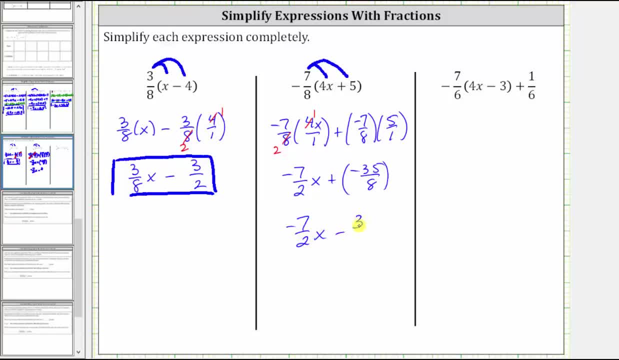 as negative seven halves x minus 35, eighths. for the last expression, we have negative seven, six times the quantity 4x minus 3 plus 1. 6th, we begin by clearing the parentheses by distributing negative 7- 6. this gives us negative 7, 6 times 4x, which is a.